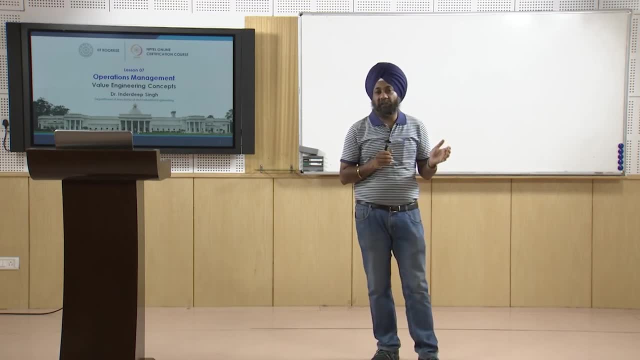 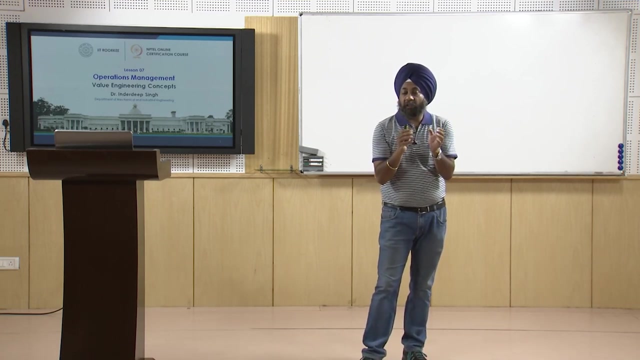 of the products have varied, or similar products have varied, or competitive products have varied over a period of time. so from that we get an idea that how is how the product sales are going to behave over a period of time. so, as a good learner, our focus must be to understand that. what type of decisions can be made by 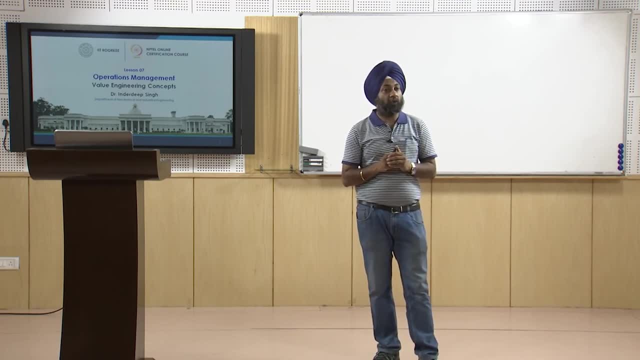 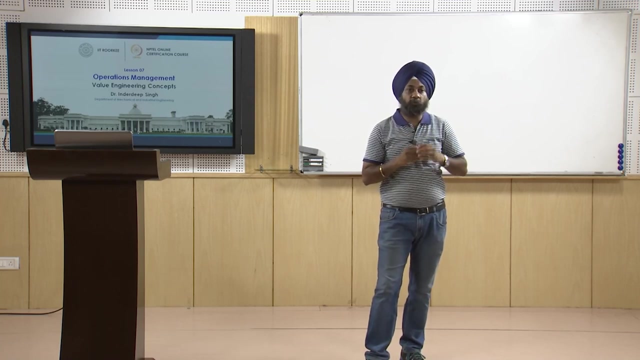 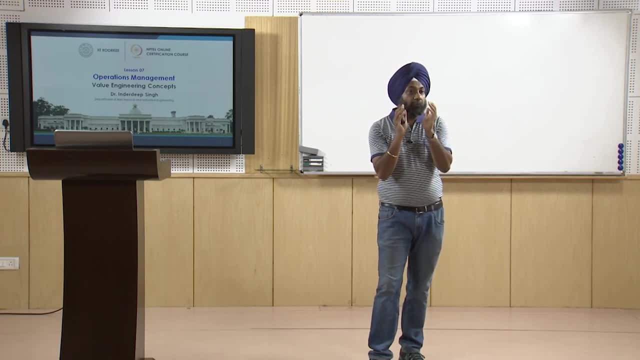 6. 76., 77., 77., 78., 79.. in ensuring a particular word, that is, value engineering, that we have information related to value engineering. also why it is important- we have seen in the previous session that new product design or innovative product design or creative product design is very, very important. 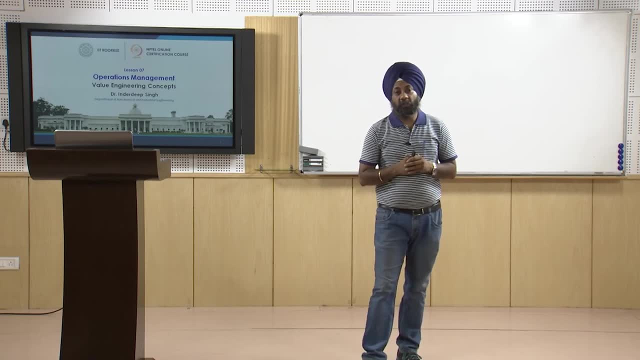 currently we are focusing on that: what the organization must produce in order to be successful. we have seen in the first week the fundamentals of operations management and now we are trying to understand that what the company must produce. then we will see may be in the next week how 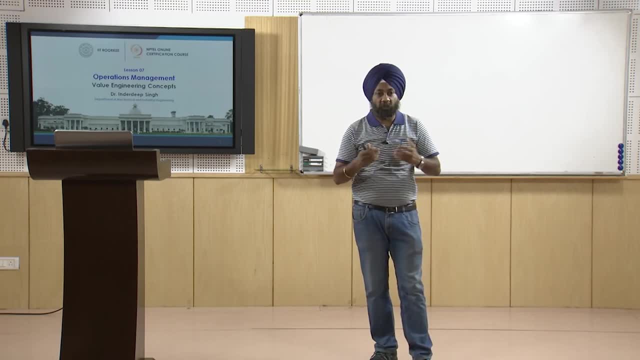 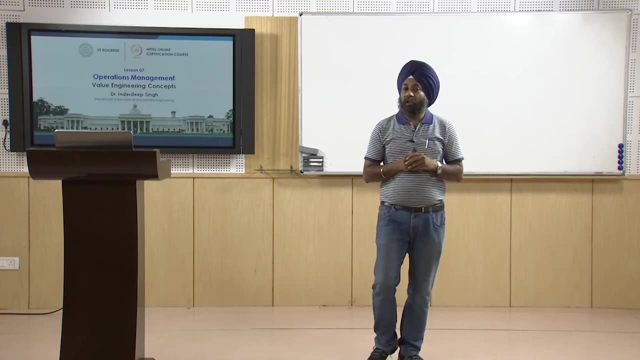 much the company must produce, that is, the sales forecasting or the demand forecasting. now, when we try to address what the company must produce, we have to answer a very pertinent question, that is, what should be our product design, what factors we should keep in product design when we are designing a product? we have recorded a complete. it was run successfully. 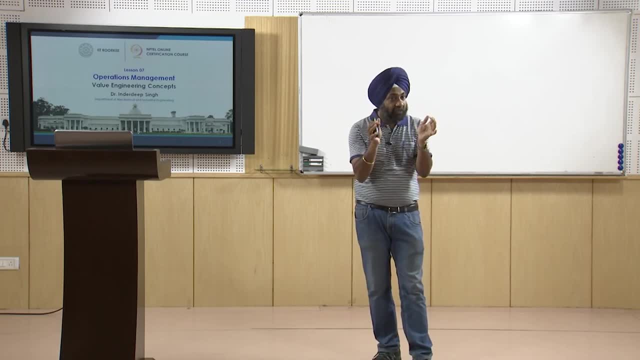 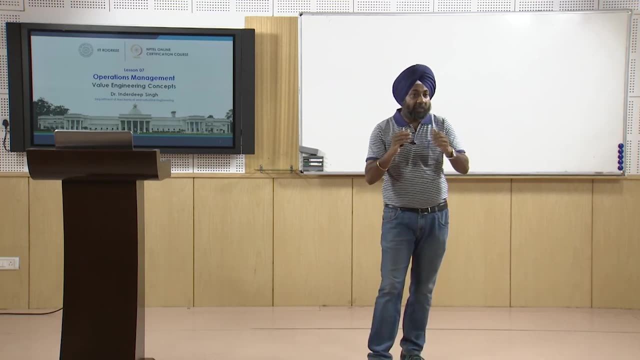 a course on product design and development, where we have addressed all these points in much more detail, but in this course on operations management, our focus is to align our students or learners in a direction in which they are introduced to a specific tools that are used for product design or the tools that help us in making a successful product design, and 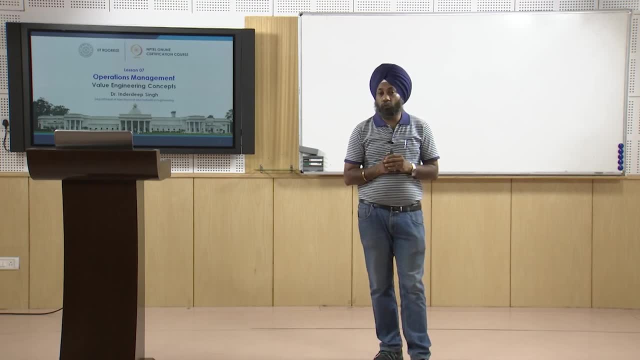 design. value engineering is what is one such tool which must be used during the product design process in order to ensure the success of the product. now, what is value engineering? what are the historical perspectives of value engineering and, sorry, what are the advantages of value engineering that we are going to cover in today's session? i must, may be. i. 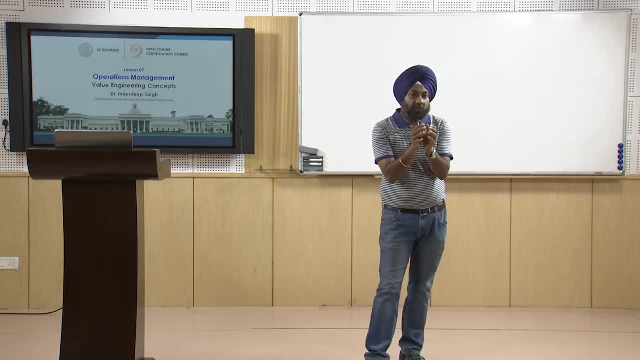 am compelled to ah make this point that value engineering is a complete course which can be taught as a thirty, five or a forty lecture course in any ug curriculum. but here we are trying to understand only the fundamentals behind value engineering, because what i see in most of the ug curriculum, value engineering is not taught as a subject, so the learners 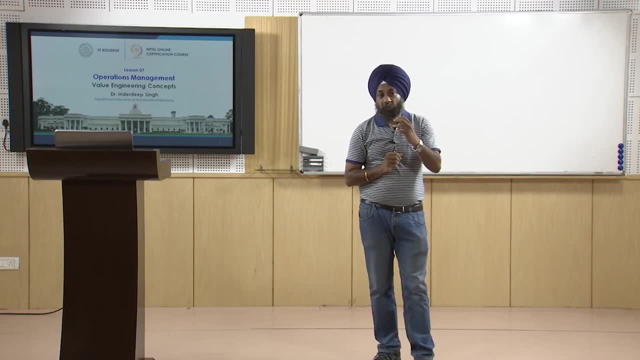 must have an idea about this wonderful concept which helps, or which has helped over the years, number of engineers and product designers to make successful products. so we will try to understand that what basically value engineering is. and we have seen that initially in the product life cycle, during the growth stage, the cost of the product is high at the maturity. 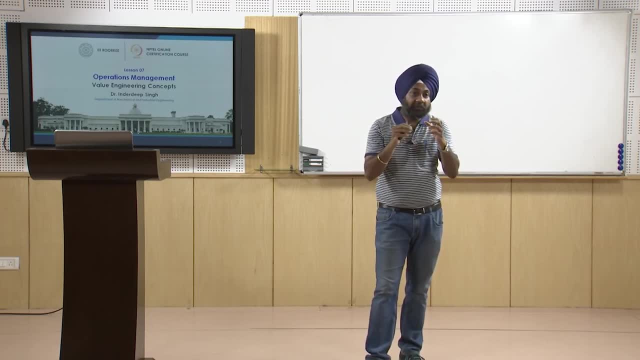 stage when the sales get stagnant. at that time the company has to focus on competition, and competition has to be ensured with cost efficiency. if you remember, in the previous session we have used this word: cost efficiency in the product life cycle. now that cost efficiency is very, very important, we have to ensure 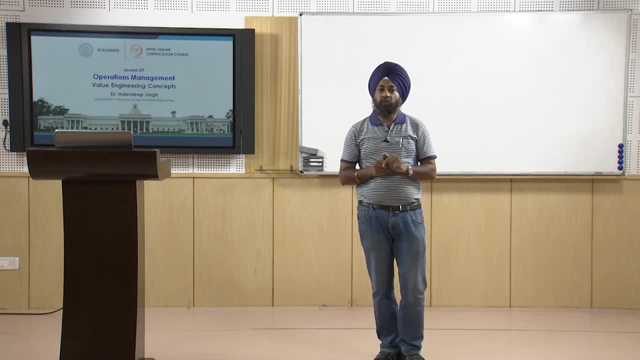 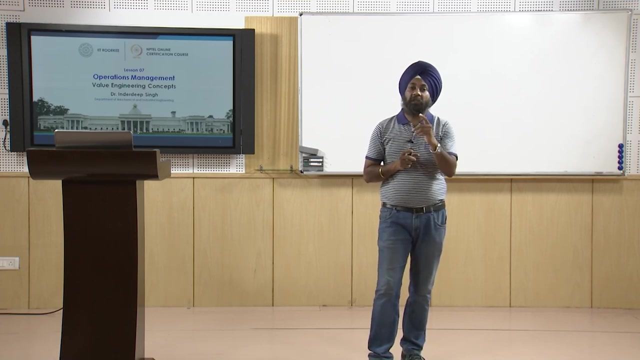 that our our product is cost efficient. our product is competitive price wise. the selling price of our product is competitive as compared to the price of the competitors product. so that cost efficiency is achieved using the concept of value engineering. now value engineering can be applied at various stages of product life cycle. now the cost efficiency is very 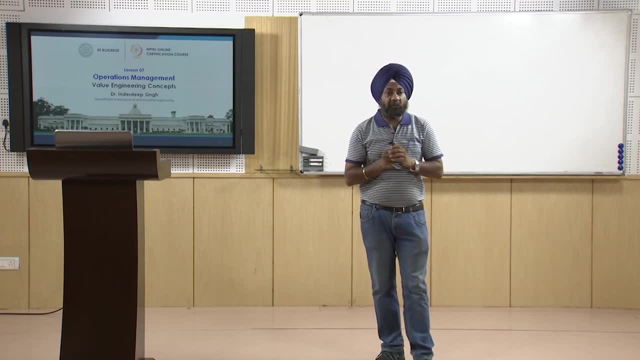 ические. the company is increasing and also theens more competitive. this means that, but also the there is a number of Bernstein- we can apply value engineering at theな price that we are getting that very high depends on the value of a product. so i am wrong. 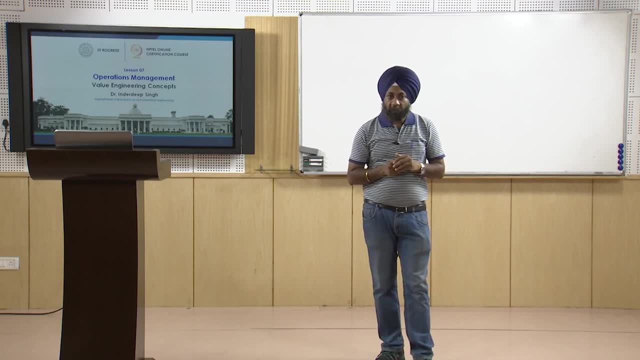 right. so here is a very good teaching that we can do it. that is why we put value engineering thisren 많. it says value engineering product plus the value engineering product is also obtained when the product ischo v, because value engineering capitalization dessert. there is no element comparing value to the manufacturing wanted system. the value engineering 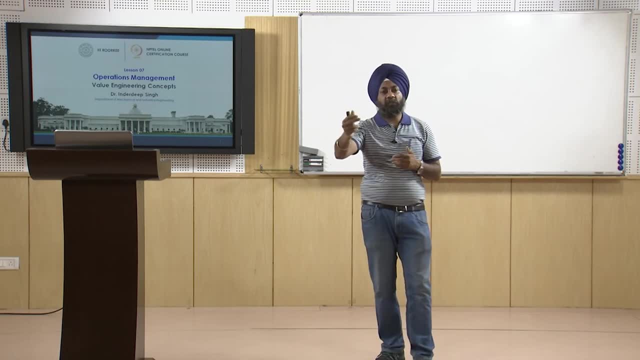 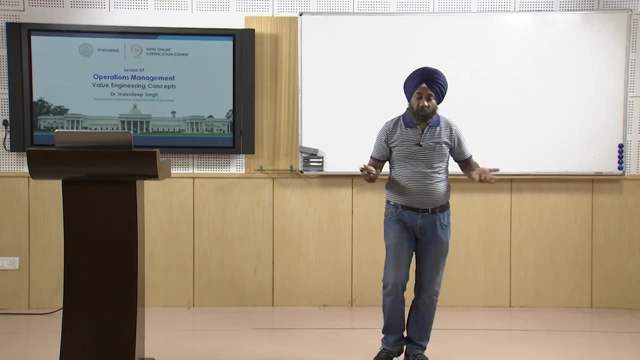 through the product on the alternative CEO. we can apply the principles of value engineering just at the start of conceptualization of a product. we can apply the principles of value engineering during manufacturing stage. also, we can apply the principles of value engineering during the marketing stage or during the logistics management of the. 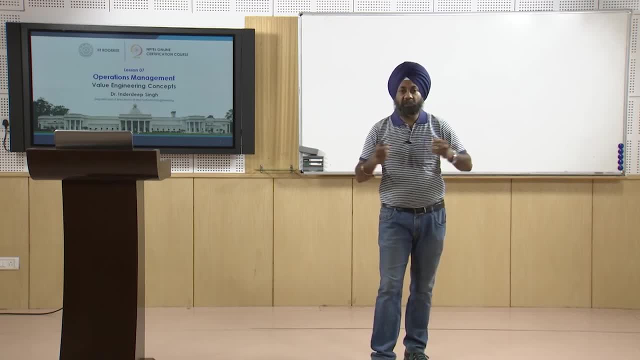 product, when the product is travelling from warehouse to the retail market. so these are universal concepts and can be applied at various stages of the product development cycle. so we will try to understand what basically value engineering is and i have already recorded few lectures on value engineering which are already available on youtube for details on 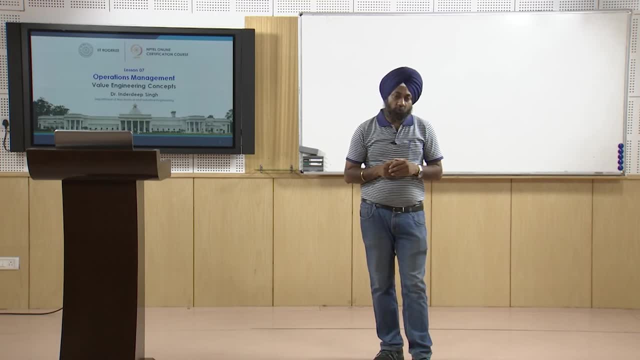 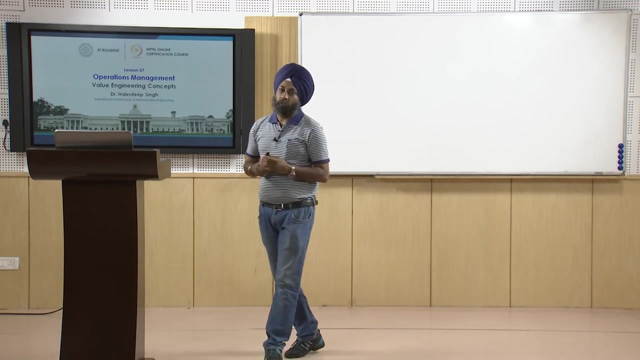 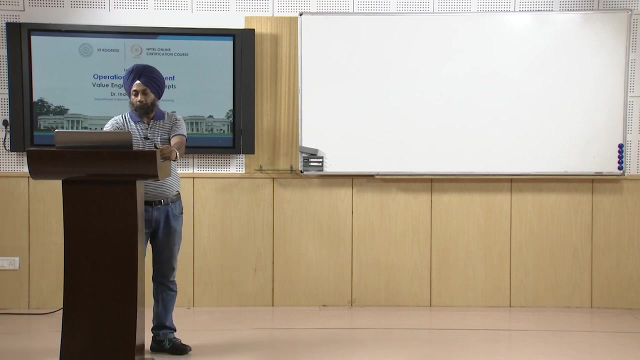 value engineering. you can refer to those lectures also, which are freely available on youtube, but today we will only try to introduce the concept of value engineering. that what value engineering actually is. so let us start our discussion with the very basic essence of value engineering, trying to understand the historical perspective of value engineering. 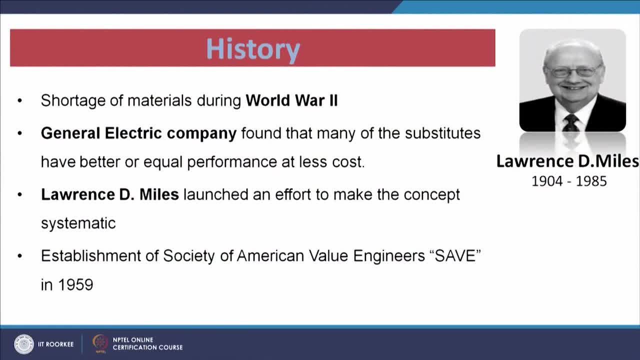 now on your screen you see the historical perspective of value engineering. so basically, during the world war two there was shortage of materials. shortage of materials in terms of repair, maintenance of the army equipment or the defense equipment. so the general electric company found that many of the substitutes have better or equal performance at less cost. now, first thing, the one word. 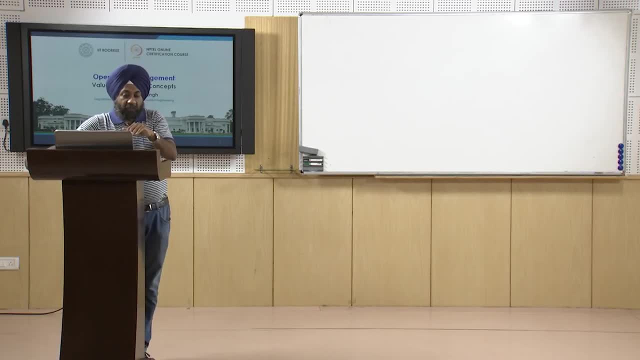 that we have to focus till now is the substitutes. there was shortage of materials. after using the materials, they revealed: lieber two 포인t. there was one complained about one part which cannot be replaced. one can that be replaced? need not replace the human, not replace the vehicle. 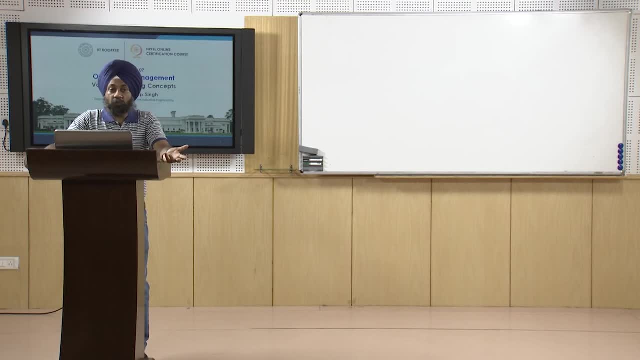 for this part, the fraternity, as you know, a insects in terms of materials, substitutes in terms of design changes, substitutes in terms of the manufacturing processes that were used for making these parts or components. And, finally, it was found out that they are equal in performance, but their cost is less. 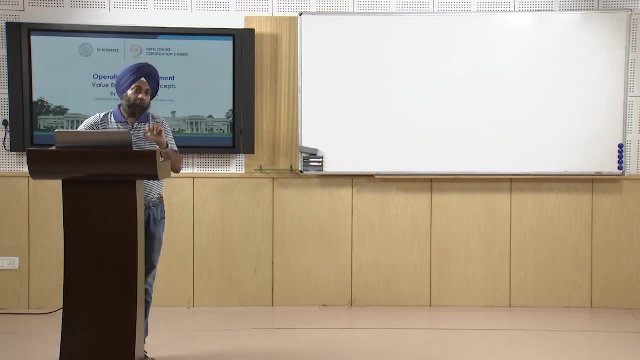 So you can see that when substitutes are used with less cost at same performance, everybody would be more than happy to adopt the substitutes. Why? Because substitutes are giving a similar performance but at a relatively less cost, And with this background this concept of value engineering was developed further. and finally, 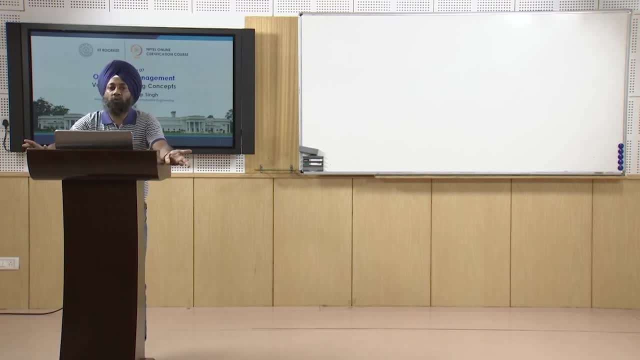 it became a completely new subject which is now taught in many engineering institutes as well as management institutes. So Lawrence D Miles- L D Miles, more popularly known as- launched an effort to make the concept systematic, So earlier it was in bits and pieces for some particular 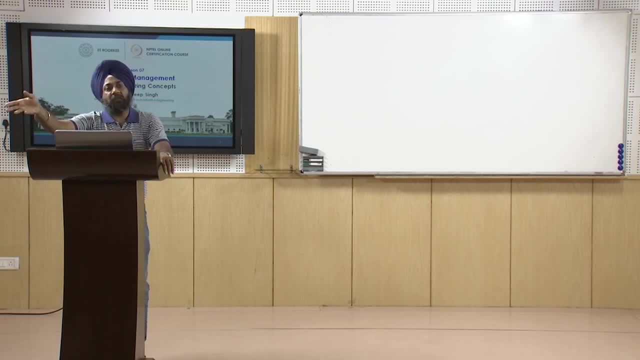 So some changes are done and then the substitute has been found to be better, or at least of equal performance. Then, in some other component, some changes were done and that was found to be better as compared to the original ones. So, finally, Lawrence D Miles thought that this is a good concept. let us make it systematic. 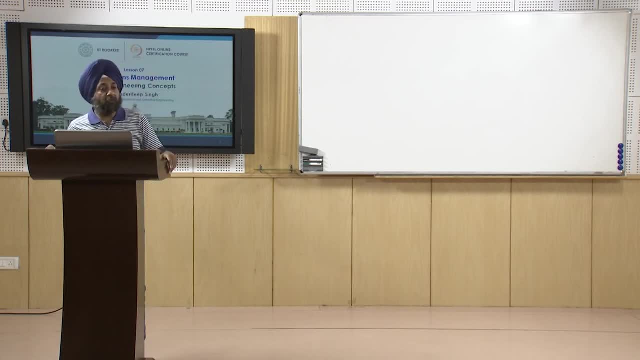 and in that process, only a society of American value engineers- SAVE, the society of american value engineers- was established in nineteen, fifty nine. so this is the background. now, i think the whole purpose of showing this slide is that what was the basic concept? the basic concept was that if you change the design, if you change the materials, if you change 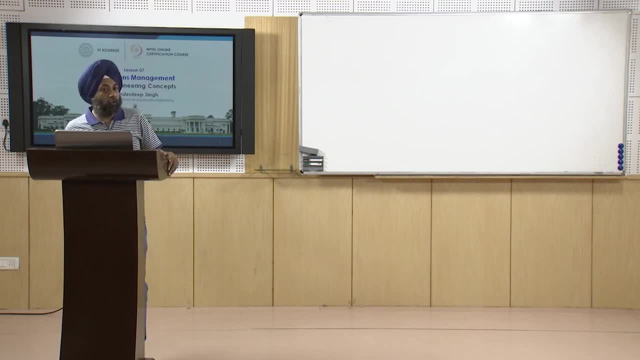 the manufacturing processes for making a particular part, component or a particular product, you may achieve a better performance, or at least equal performance, but at a relatively lower cost. so the performance has to be same but the cost is lower. so that is the basic concept behind value engineering. when i first heard of this term, value engineering may be ten. 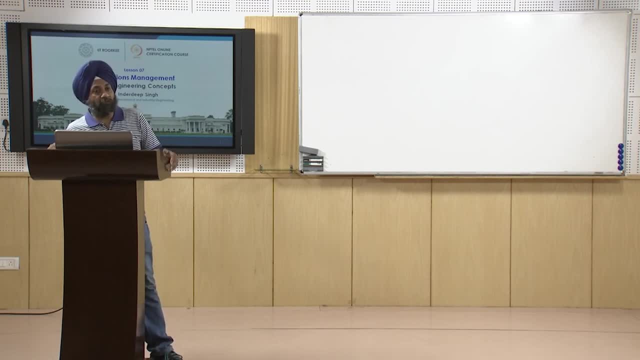 years back i thought this topic has to do something with the moral values, and that is what the most engineers think about value engineering. you may achieve a better performance or at least equal performance, but at a relatively lower cost. if you ask somebody what is value engineering, many engineers will not have an. 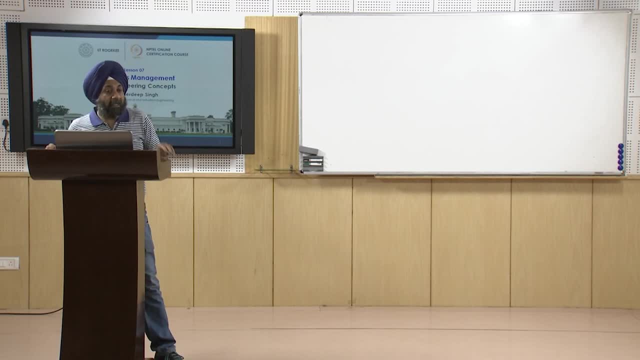 idea that what value engineering actually is. but after this session or after attending various other sessions which are freely available on electronic media, you can very easily try to understand this concept. and the basic concept is- again i am highlighting- we have to ensure the performance by change in materials, change in processes, change in design. 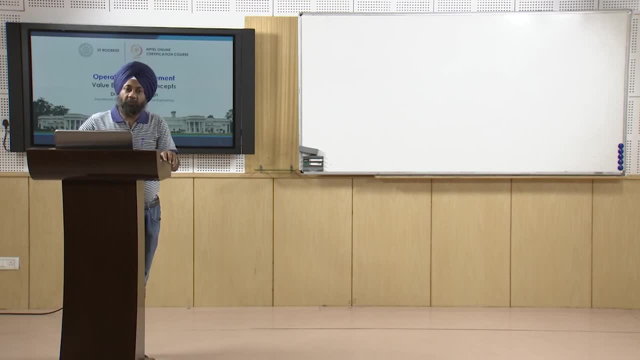 and then change in process. we can decide the detail without compromising the cost part may be. we have to focus on the cost also. we have to ensure the performance, ensure the function is achieved but at a relatively lower cost. so that is the basic concept of value engineering. we will read one or two definitions also today, but the theory part maybe explained. 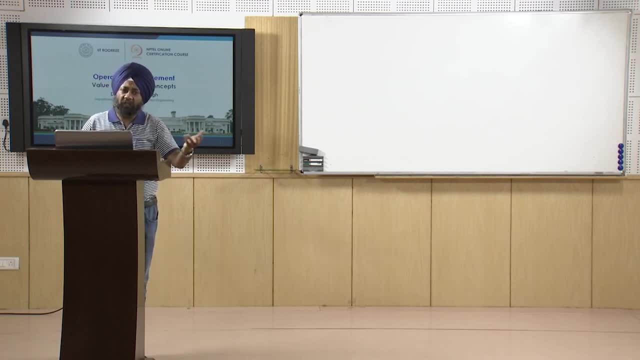 or can be understood from different text books and from different other media, but basically basic understanding that what value engineering actually is must be clear to the learners. now, what value engineering is? i have tried to explain what is not value engineering. that also we need to understand now. value engineering is not cost cutting. some of you may be wondering. 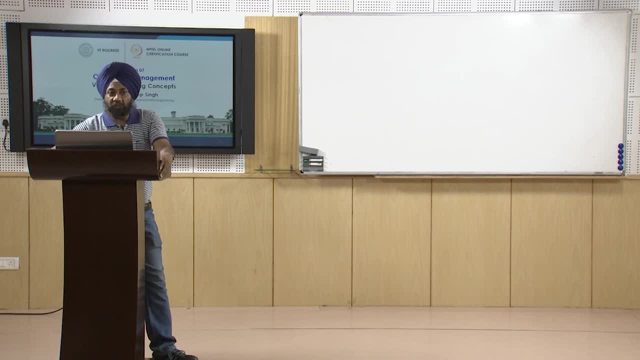 that we are reducing the cost of the part or the component. therefore, it is cost cutting. no, in cost cutting we sometimes compromise on the quality, on the performance, on the serviceability, on the maintainability, on the reliability of the product, but in case of value engineering, we are not going to compromise on any of these aspects. the performance of the product has. 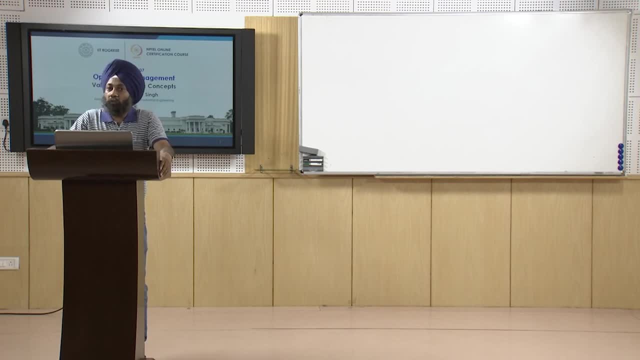 to be ensured. we have to ensure that the product that we are designing must be reliable, easy to service. it should be easy to maintain life cycle, cost should be low. so we have to ensure everything in value engineering, but still we focus on reducing or minimizing the cost of the product. so therefore, there is a difference between cost cutting and value. 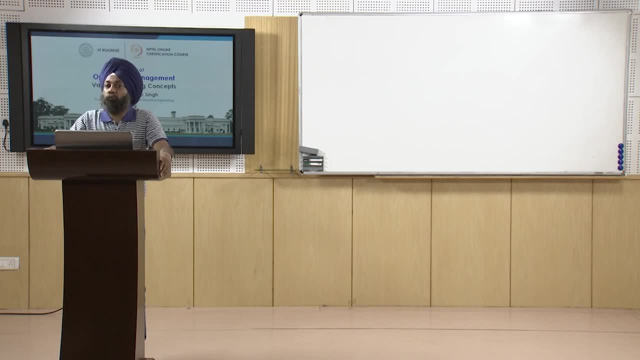 engineering. value engineering is more design focused. we will try to achieve the function at the minimum possible cost, whereas in cost cutting we just look at producing the product in a way that the cost gets reduced. so, design based value engineering, manufacturing based cost cutting. in cost cutting we may change in cost. 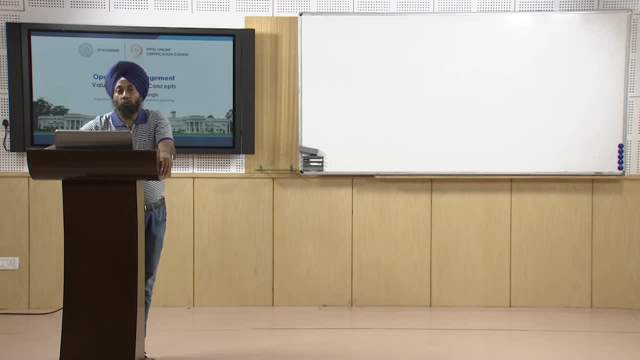 cutting. also, we will look for alternate materials, we will look for alternate processes, we will look for alternate designs. but in cost cutting the focus on alternate designs is minimal, whereas in case of value engineering, we will only focus on design and we will see that. what is what the design modifications can be done. in order to ensure that our function is achieved. so value engineering is design based. cost cutting is production or manufacturing based, where we focus on reducing the cost or cutting the cost of the product. so cost cutting and value engineering is very, very different, and you must be able to answer a very simple question, that: what is the difference? 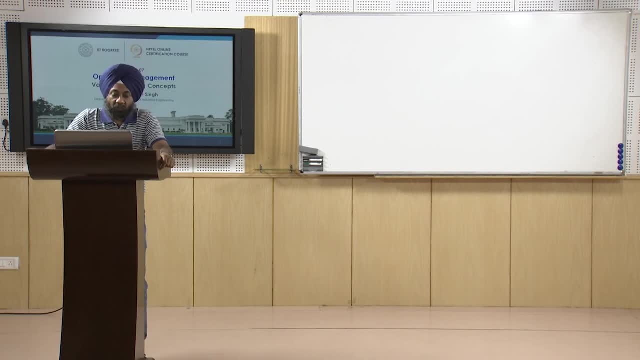 between value engineering and cost cutting. then some people say that value engineering is design review. now, from these two words, design review, very literal meaning comes to me: that once, first we design and then we review it. no, the this is not design review. we will use the concepts of value engineering during that design process itself. we are not going 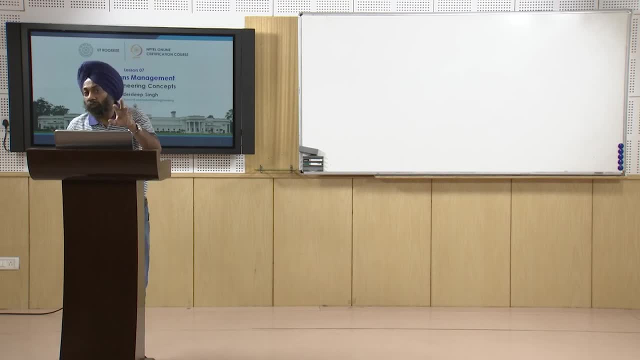 to review the already designed product. we are going to focus, focus on the design, only that, what should be the ideal design for this product, or what should be the ideal design that will satisfy the desired function. For example, the function of this wrist watch is to show time. usually, if you go into detail, 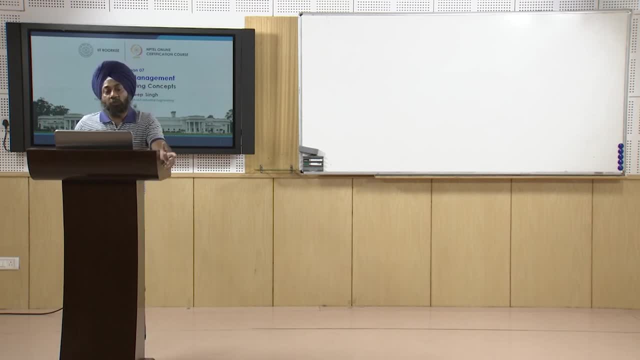 of value engineering. for identifying a function, usually we use a 2 word, verb, and a noun definition. Now verb and noun definition means verb is show time, is noun, So we use verb and a noun type definition. that is show time for a shaft. it can be transmit. 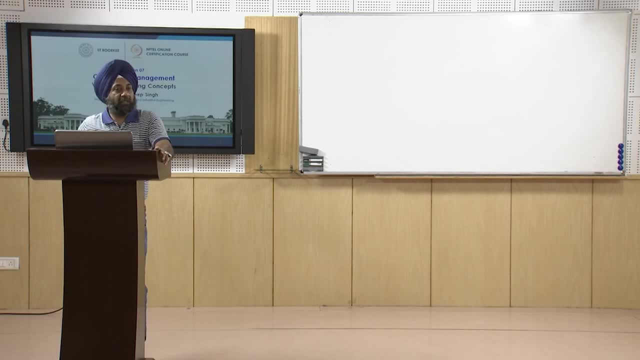 torque. for a fan it can be circulate air. for a newspaper it can be provide information. So for different products we will have a 2 word verb and a noun type of a definition. So we will try to see that when we are designing a product. 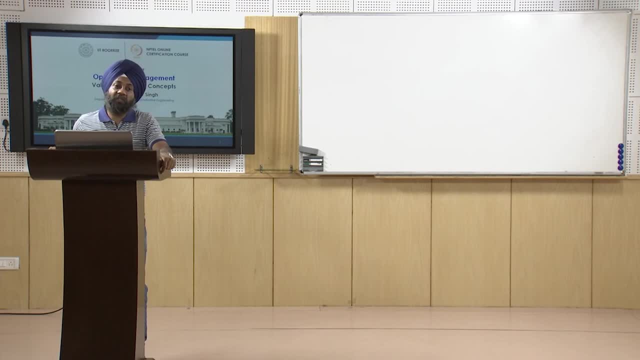 How the principles of value engineering can be used to achieve the desired function. Now, desired function. I have already told you that for this wrist watch, the desired function can be show time. Now I have to ensure that whatever product I design, it should be able to satisfy this. 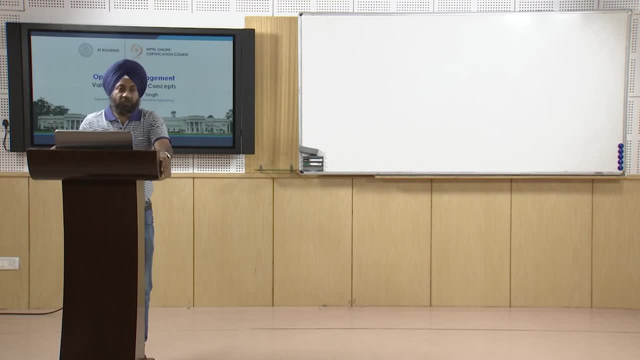 function of showing the time. I will not start my design from this watch. I will start my design from the basic, Basic function, that is, show time. So this wrist watch is completely ruled out. I will think I will use my creativity to design a product which will satisfy this basic function. 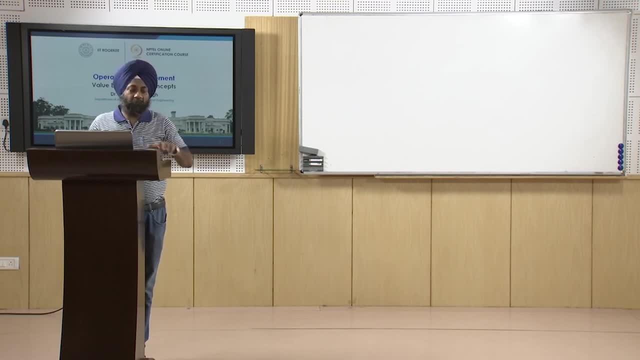 of showing time. It can be a completely new design completely eliminating the use of the wrist watch. whereas in case of cost cutting, I will just take this watch and try to see that how I can change the dial, How I can change the various components of this watch. 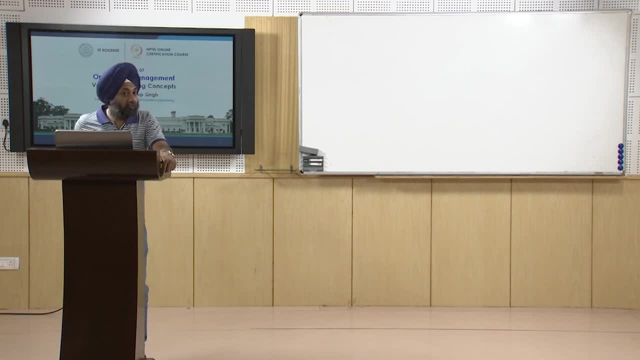 So that the cost gets reduced, whereas in value engineering, I will focus on the design of a product in such a way that the use of this band and this watch is completely eliminated and I am still able to satisfy my desired function of showing the time or seeing the 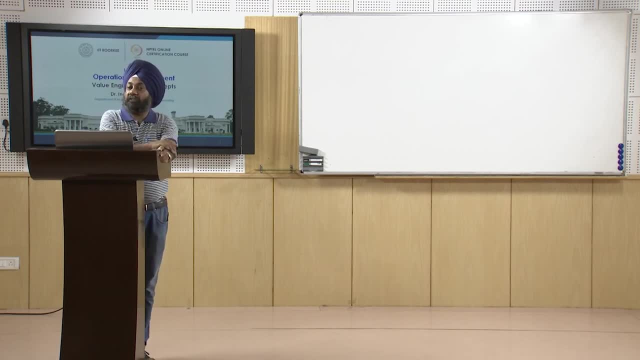 time. So during the design only we will focus that: what is the desired function and how it can be achieved with modification in the design, See Simultaneously ensuring that the cost is also minimal. Similarly, a value engineering is not project elimination, So we are not going to eliminate any projects, or it is not a criteria for evaluating the 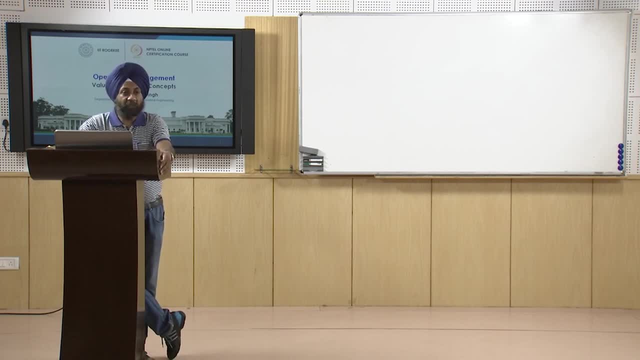 projects and then eliminating those projects based on value engineering. No, it is not project elimination, It is not scope reduction. Many times people feel that if you use a value concept of value engineering, the overall scope, scope of the product will get reduced. No, the scope of the product may further increase. 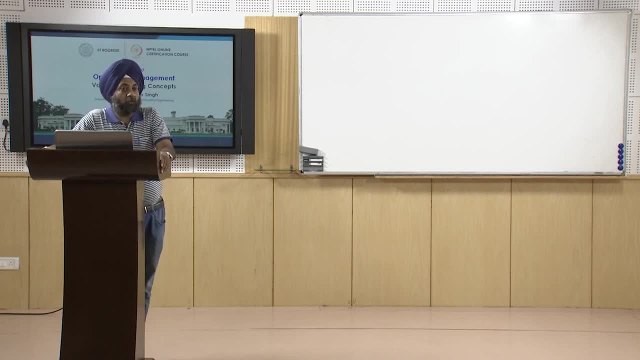 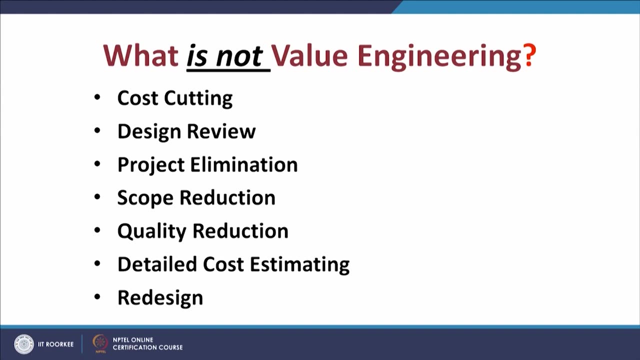 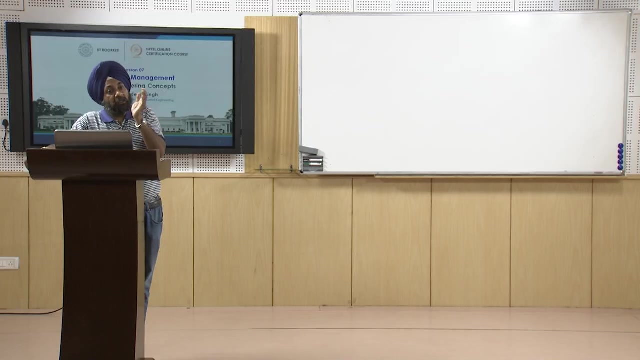 Quality reduction. I have already told we are not going to compromise on quality when we are using the concept of value engineering. Similarly, this is not detailed cost estimation, So we are not going to do cost estimation Definitely. we are going to see what is the cost of the new design. what was the cost? 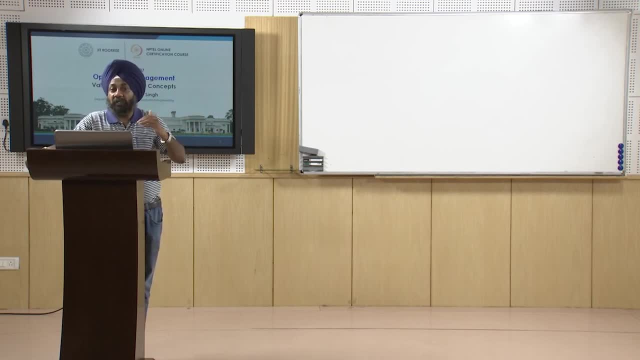 of the old design Whether we are saving Some cost. in many cases the cost may further increase also, but the overall performance of the product is increasing. So it is not cost estimation, It is the design philosophy in which we design a product in such a way that our intended 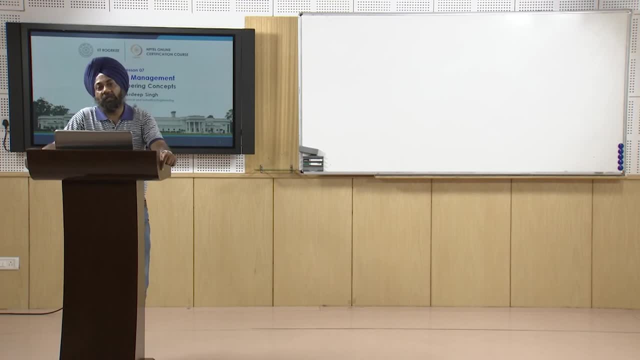 function or the intended function of the product is satisfied at the minimum possible cost. So it is not only a cost estimation technique, It is basically a design tool which helps us to focus on the basic function of the product. Okay, And try to achieve that function at the minimum possible cost without compromising the quality. 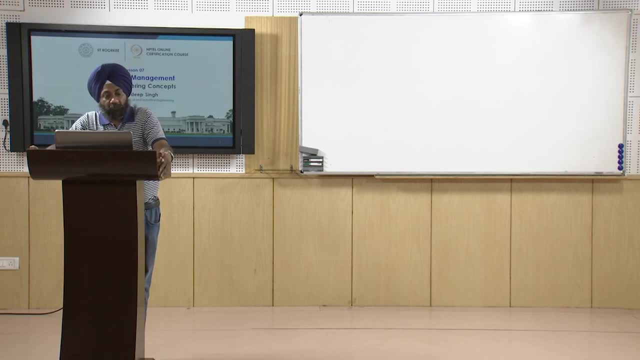 performance, reliability and serviceability of the product. Moreover, it is not redesign. It is a design tool which can be used by the engineers. Now I think, with this background, let us go through one or two definitions of value engineering. What is value engineering? 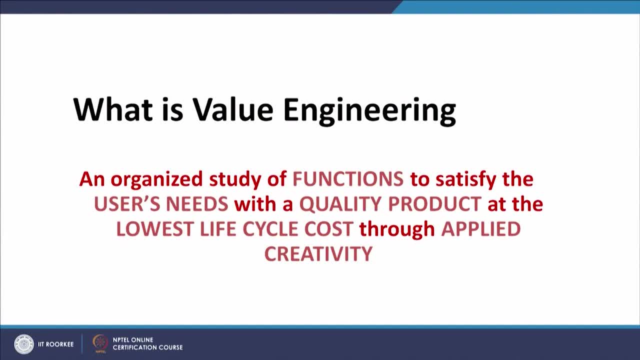 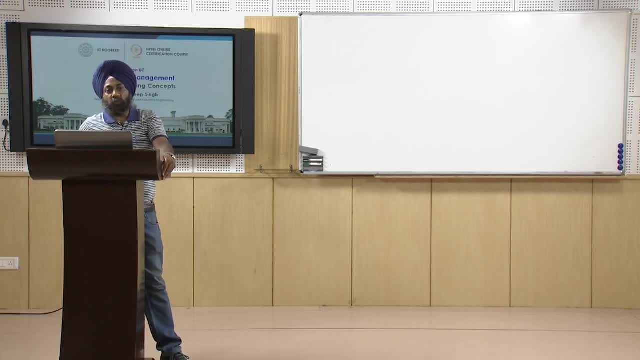 On your screen you can see An organized study of functions. Now all of you know function I have told. the function of this wrist watch can be show time. The function of this tube light can be illuminate the illuminate room. The function of glass can be store water. 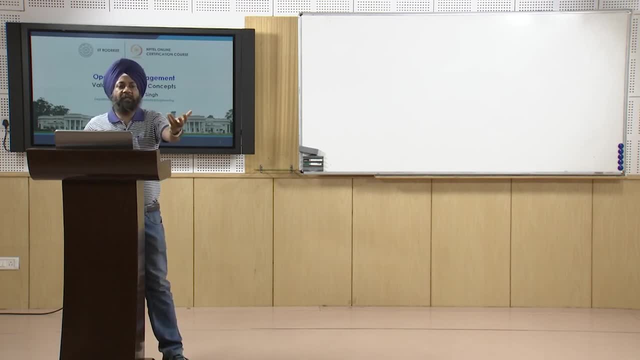 So you have, you can see products around you and you can identify the function of the product. Now, value engineering is an organized study of functions. Why do we need to study the functions? To satisfy the user needs. Now I am using this wrist watch. 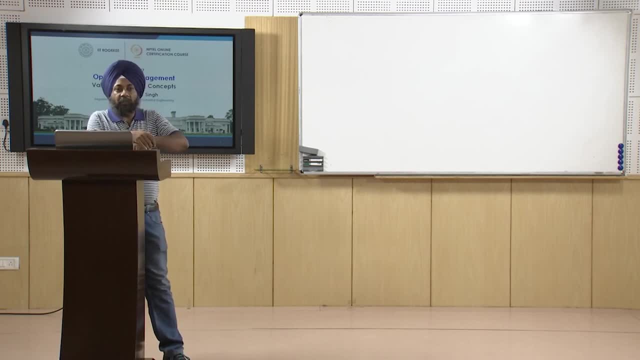 I am the user, my what is? what is the function for which I have bought this watch? I want to see time, So I have that. find the watch should satisfy the users need. It is satisfying my need. I am able to see the time in this watch. 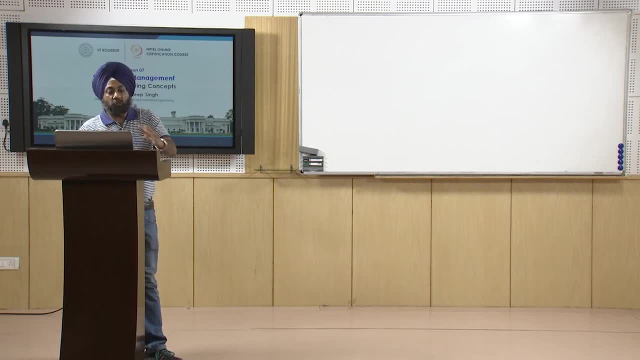 So an organized study of functions to satisfy the user needs With the quality product. no compromise on quality, At the lowest life cycle cost, yes, without compromising the quality. cost should be less through applied creativity. Now, how that is possible? we have to use the creative juices of our mind or of our brain. 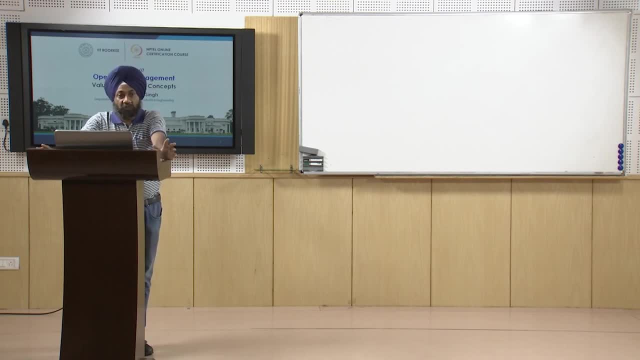 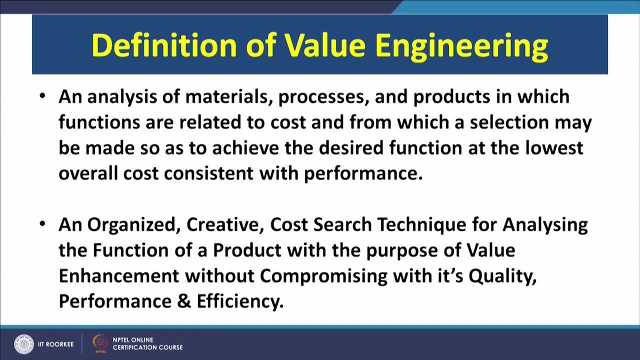 to come up with modified solutions. So this is the basic concept of value engineering: To satisfy the user needs, To satisfy the desired function reliably, at minimum possible cost. These are the other definitions of value engineering. ah, I will just read these definitions for you. 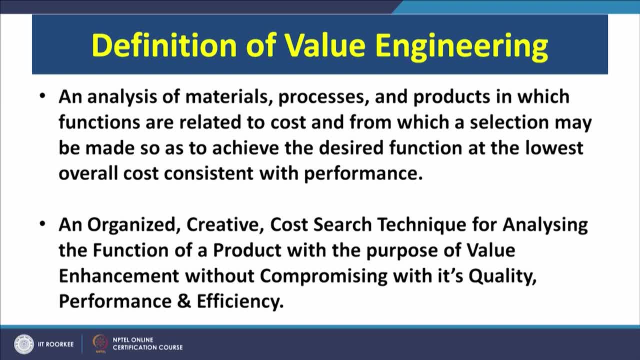 An analysis of materials, processes and products in which functions are related to cost and from which a selection may be made so as to achieve the desired function at the lowest overall cost consistent with performance. So I have already explained everything related to this definition. Another definition can be: it is an organized, creative, organized, systematic. it is not may. 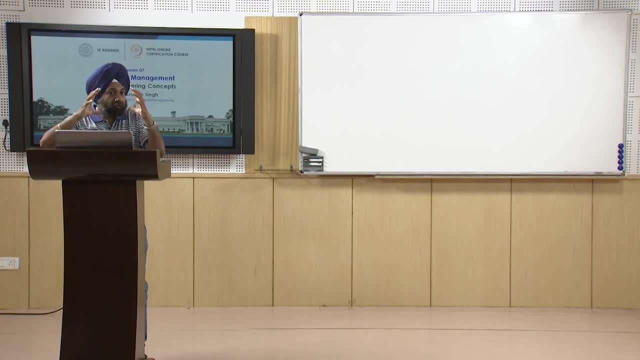 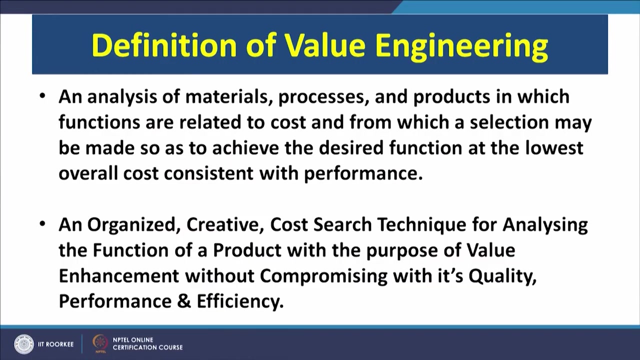 be haphazard or philosophical. it is organized step by step approach. it is systematic approach and organized creative cost search technique for analyzing the functions of a product without the purpose of sorry, With the purpose of the product, With the value are length enhancement without compromising with its quality performance. 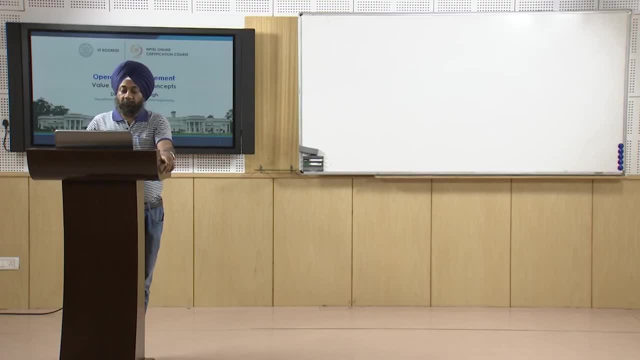 and efficiency. Now, what is the purpose of purpose is enhancement of the product, the quality of the product. so purpose of value and hence method of our you can be directly proportionate to the quality, reliability, weight reduction or efficiency. now what is our focus in value engineering? 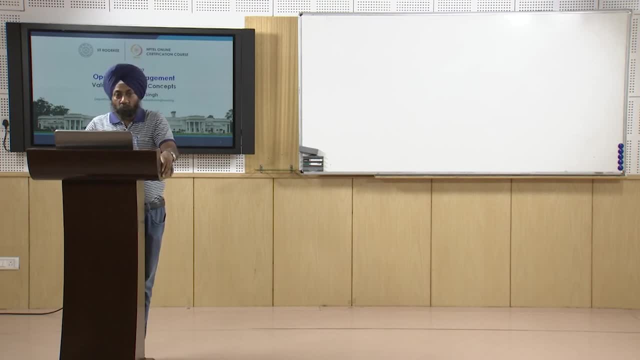 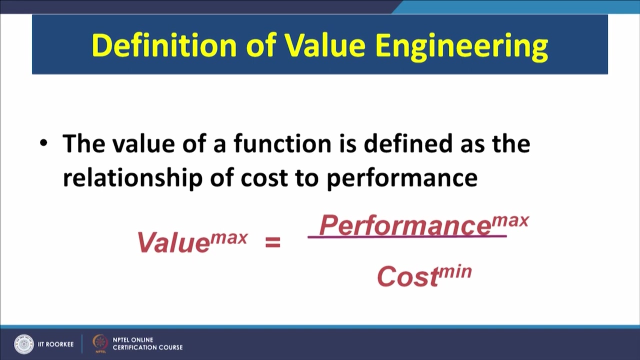 and enhancement of the value of the product without compromising it with the quality, performance or other parameters of value. mathematically also, the value of a function is defined as the relationship of cost to performance. so we need to maximize the value on your screen, you can see. we need to maximize the value, performance and cost. 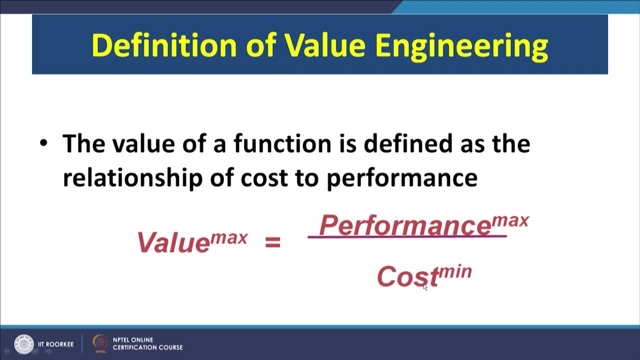 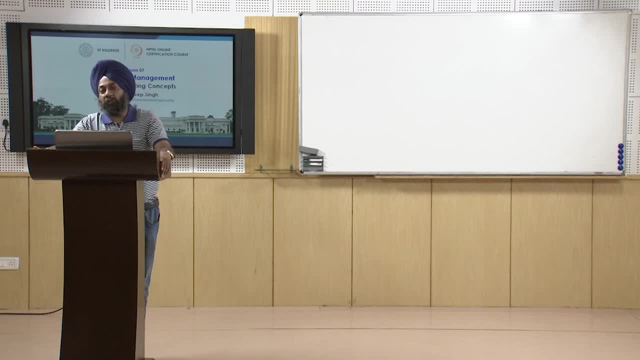 are two things that we need to take care now. value is directly proportional to the performance and inversely proportional to the cost. so if the performance of the product is increasing, value is automatically increasing. if the cost of the product is reducing, the value is automatically increasing. so therefore we see that enhancement of value at a lower cost or by increasing. 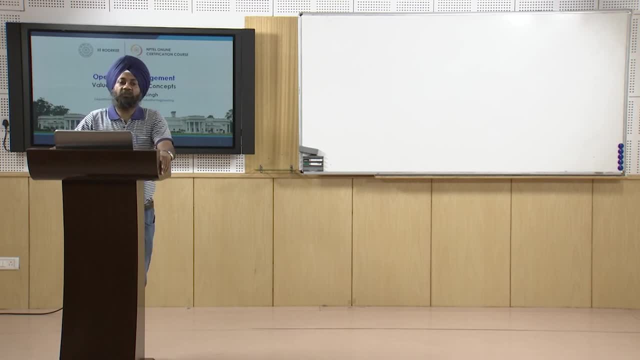 the performance of the product. both ways can enhance the value. many a times it may so happen that the performance is remaining unchanged, but the cost is reducing. still the value of the product increases. sometimes it may so happen that the performance is increasing but the cost is remaining same. still the value. 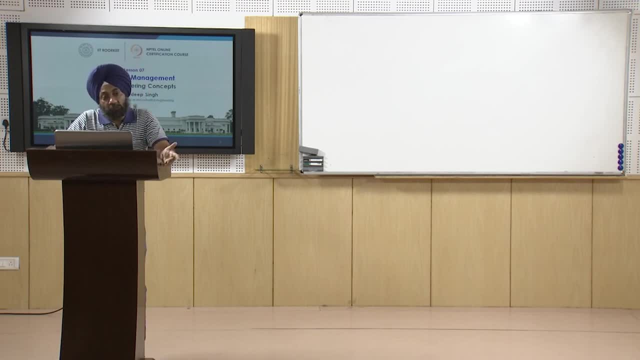 is increasing. in the last case, it may also happen that the performance is increasing. at the same time, cost is also increasing, but the relative increase in performance is much more than the increase in cost. still, the value is increasing. so we can adopt different strategies to ensure that how the product value can increase or how the product value 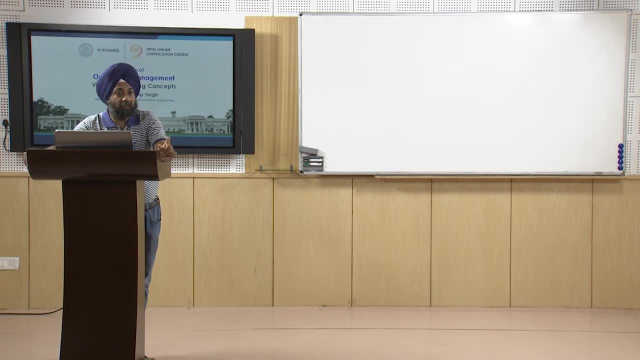 can be enhanced, and that is the- you can say- place or situation wherever creativity will come into picture. we can come up with different solutions of increasing the performance or the functions of the product without changing the cost or by reducing the cost. Now lets see what are the solutions for increasing the performance of the product by changing. 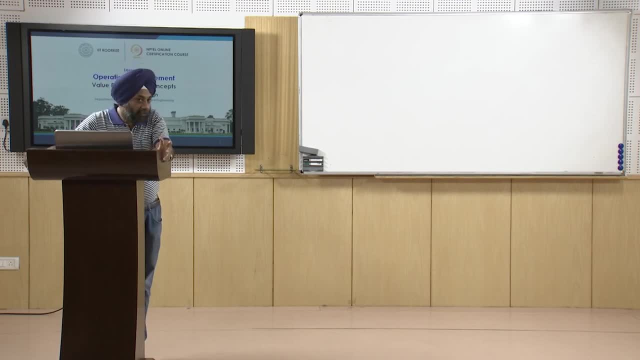 the cost, reducing the cost. So that is the major. maybe if today's lecture you want to summarize or you want to just remember one particular thing from today's session, that is, value is equal to performance by cost, or value is equal to function by cost. 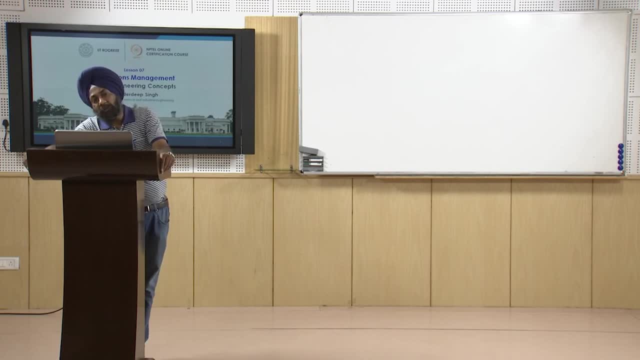 We need to maximize the functions and we need to minimize the cost, or we need to maximize the performance and we need to minimize the cost. So this equation can be helpful to you for understanding the basic concept of value engineering. Now why there are poor values in the product. 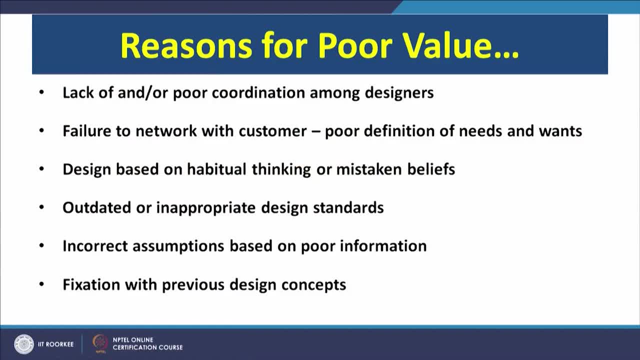 I will just read these points for you: Lack of poor coordination among designers, failure to network with customer, poor definition of needs and wants. So sometimes you see different products all around you And you find out that this product could have been designed in a better manner. 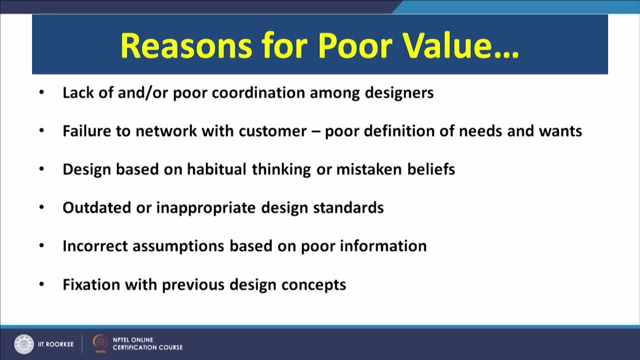 But why this has not been designed in that particular manner? These are the reasons. there is lack of coordination among designers and then the design is based on habitual thinking or mistaken beliefs. Many times we just follow. change is always not welcome by engineers or scientist. 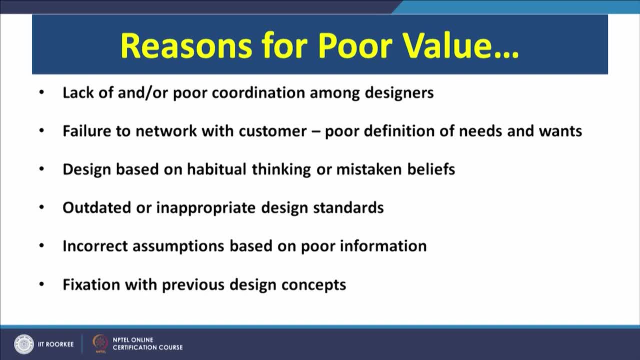 Many times we are doing a particular thing, we are using a particular algorithm, we are using a particular process. We follow. we want to follow the same procedure, we do not want to change. So design is based on habitual thinking. definitely, it may not be the best design which could. 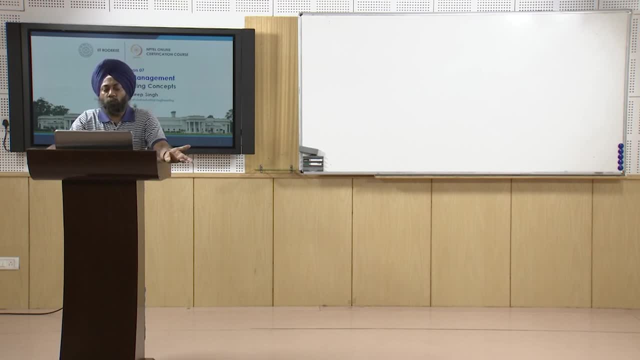 be done to satisfy that function. Outdated or inappropriate design standards. there are number of design standards which have become completely outdated in today's scenario, but still many designers focus on those design standards only Incorrect or inaccurate assumptions based on poor information. Sometimes designers or engineers do not have the latest information and therefore they 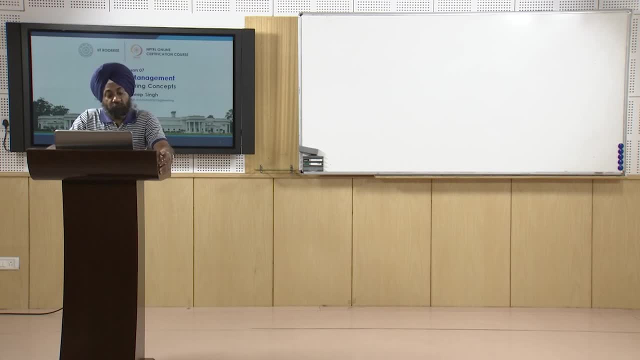 design the products with whatever information they have and fixation with the previous design concept. So, basically, the summary is that our designers need to be innovative. our designers need to be creative, they need to shed their inhibition, They need to get away from the already established methodology of product design in order to 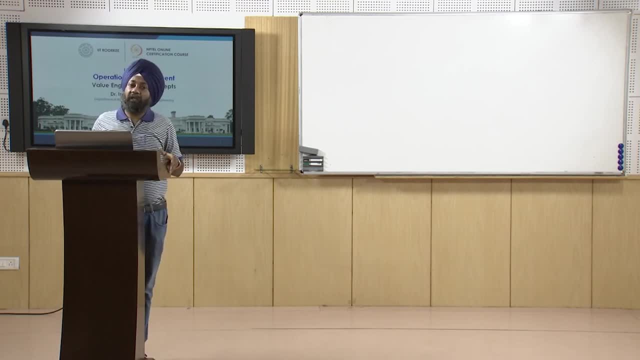 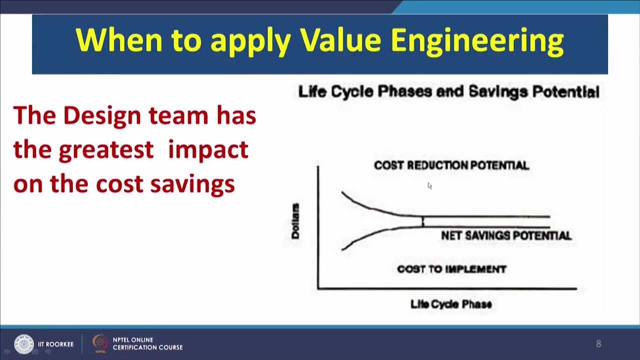 design products Which can satisfy the function at a relatively lower cost, and there the value engineering and the creativity comes into picture. Now, when to apply value engineering. If you see the cost reduction potential in the graph, The cost reduction potential is coming down as a life cycle phase is are increasing. 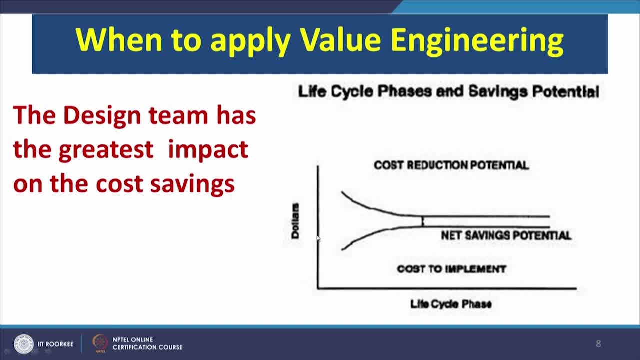 So during the design stage only, the saving potential is more, because everything is fixed at the design stage: The shape, the weight, The material, The training, The factors, The management, The type of the how, these, indeed, How are they day to day maintaining? 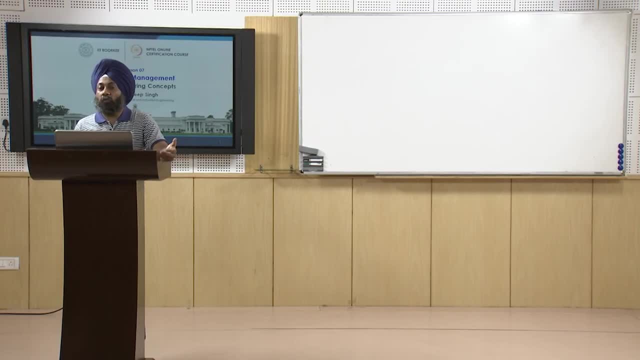 materials, everything is fixed at the design stage. So the cost reduction potential is maximum at the design stage. So the design team has the greatest impact on the cost savings. Then the question is that when we must apply the concept of value engineering, we must 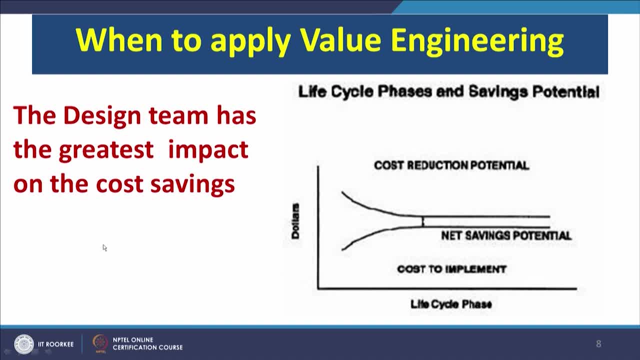 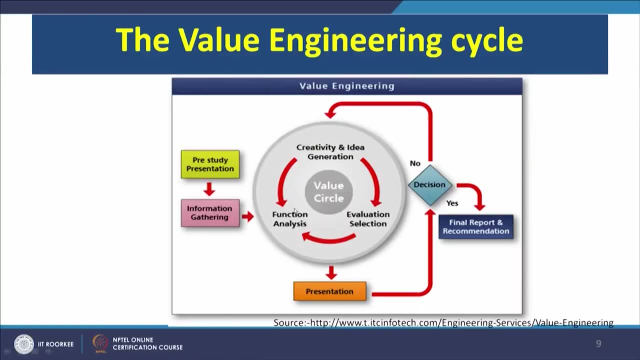 apply the concept of value engineering during the design stage of the product and therefore we are covering value engineering in the product design and development process. This is value engineering cycle. it is available on Google images. So creativity and idea generation is the backbone of value engineering. 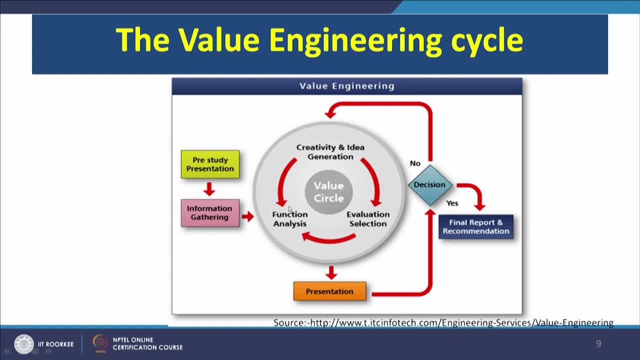 Then we do the evaluation and selection of the ideas and then we do the functional analysis that whether the desired function that the customer wants is achieved by our idea or not. If it is achieved, Then we go further and we do the final report and recommendation. 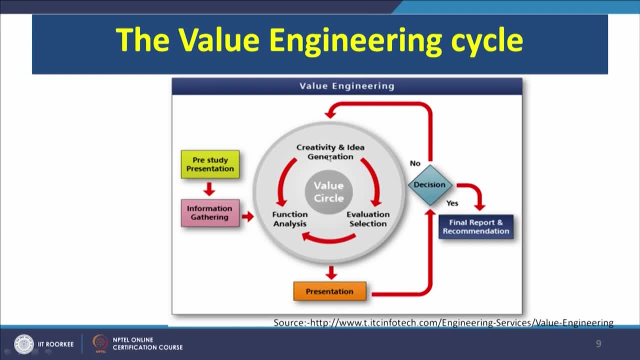 So maybe this is the value circle: creativity, idea generation, evaluation, functional analysis and, finally, the decision whether the product will be successful or whether the idea can be taken further for developing it into a tangible product or not. Now, what are the application areas? 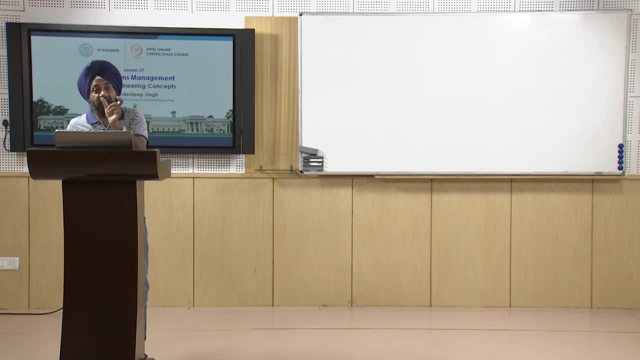 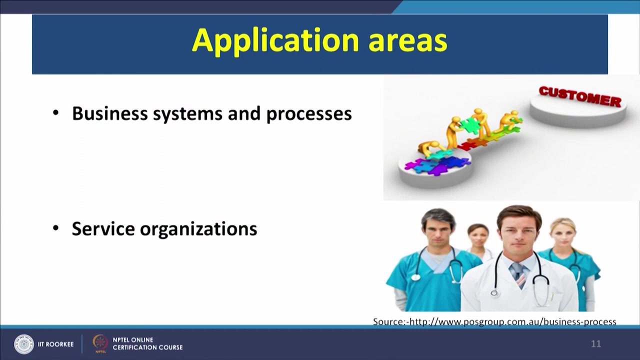 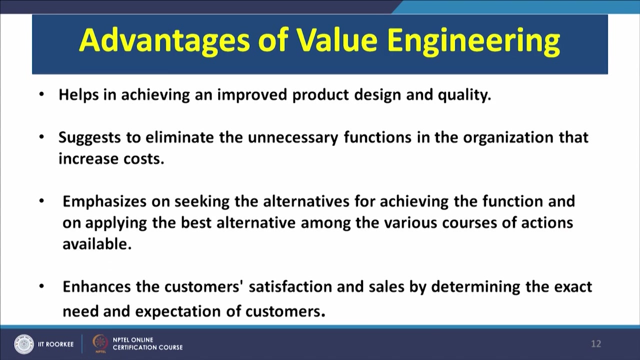 Value engineering has been- I am applying Value engineering has been successful in construction projects. It has been successful in manufacturing industry or manufactured products. In business systems and processes also, the concepts of value engineering have been found to be successful, as well as in service organizations. 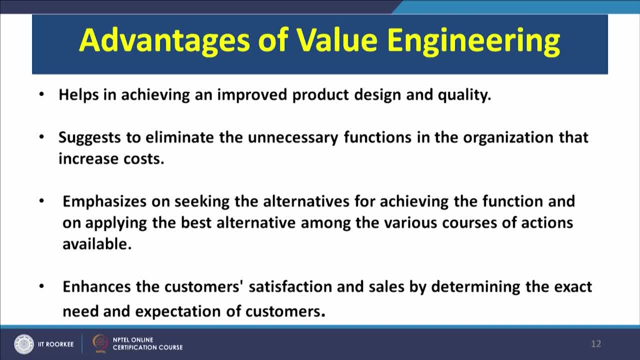 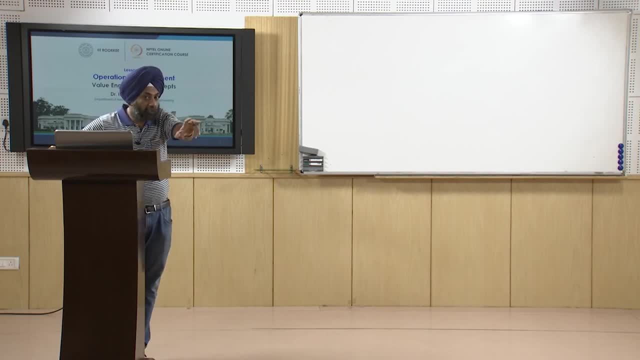 Now, what can be the advantages? let us quickly understand. It helps in achieving an improved product design and quality. So what are the advantages? So we are able to design a better product if we use the concepts of value engineering. because now we are focusing on the basic function and we are trying to understand that. how this? 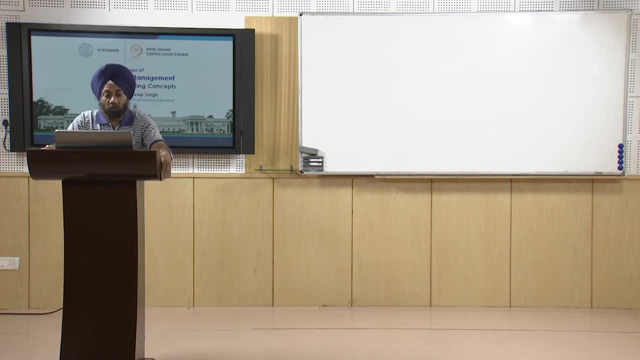 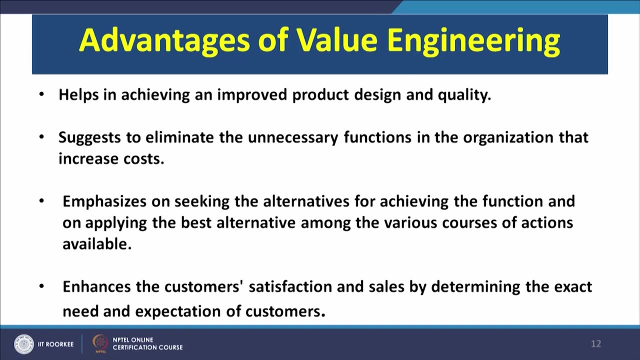 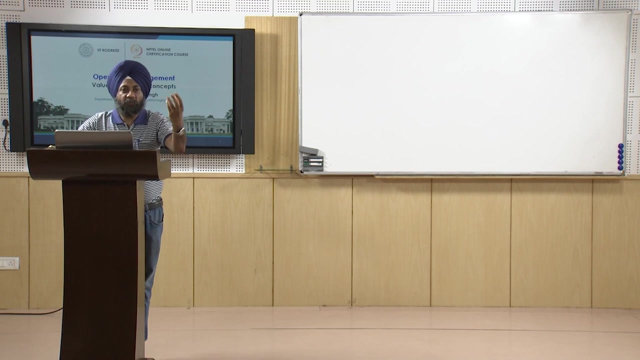 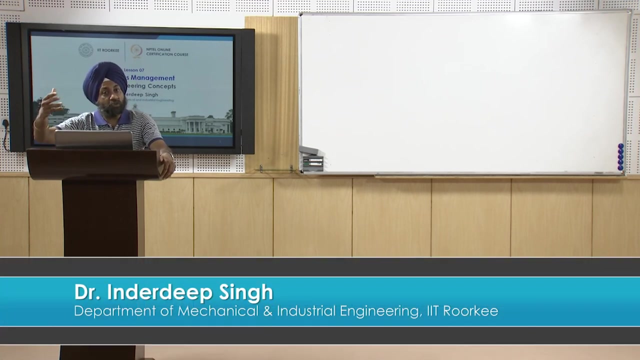 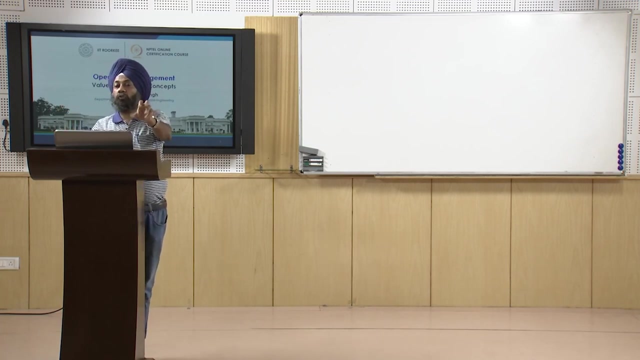 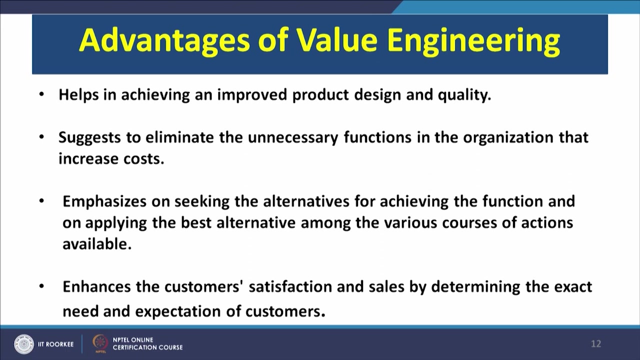 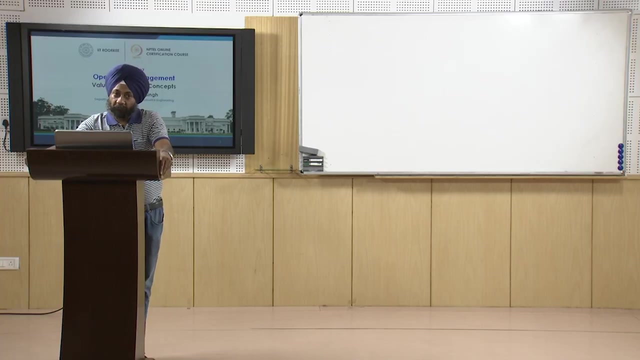 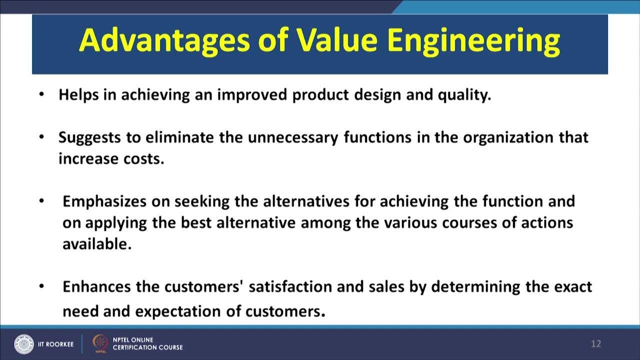 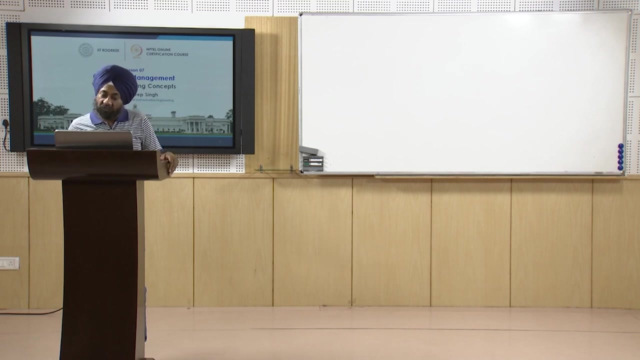 function can be achieved reliably at the minimum possible cost and it suggests to eliminate the unnecessary functions in the organization. that increases the cost Not only in the organization, in the product also. if you see, all of us use mobile phones, smart phones. We are able to design a better product design into account while designing the product and 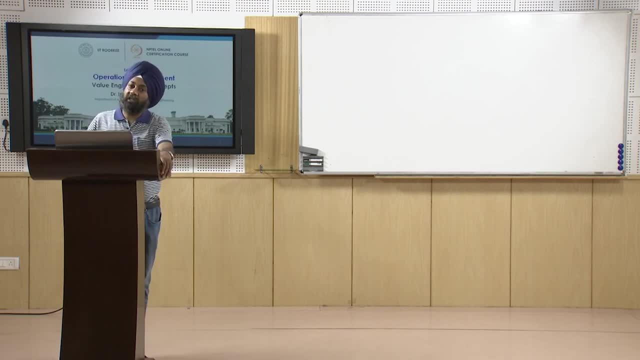 then we focus on the desired function and we try to achieve that desired function at a minimum possible cost. So I think with this we will end today's session. I have tried to introduce only the concept of value engineering, and that is very, very relevant concept. during the product design process and value engineering- most of the 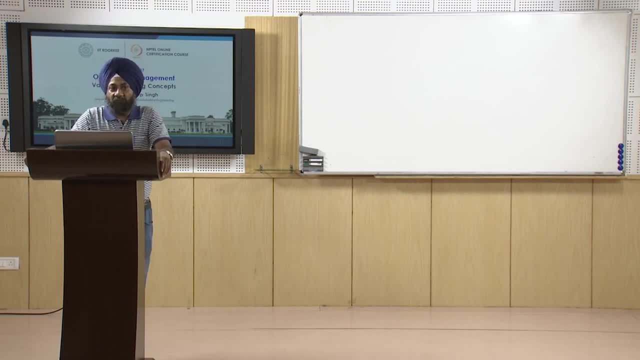 times is not covered in the product design. It is not covered in the product design and development chapter. So, therefore, we thought of introducing this tool to the engineers or the learners, so that engineers can further enhance their skills and focus on the product design, keeping in 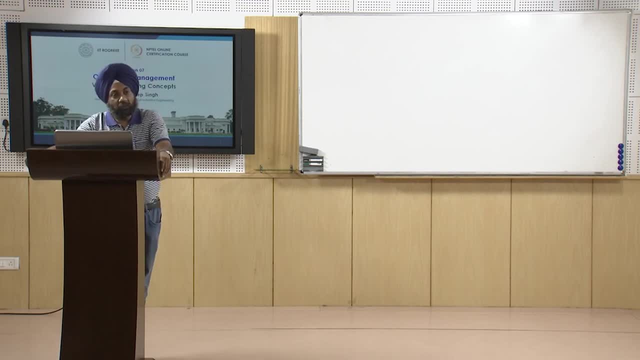 mind the concepts of value engineering, and further information is available on various other sources. So I request all the learners to look up for other sources and improve or increase their know how in this important aspect. Thank you, In our next session we will see another aspect that is very, very important that we usually